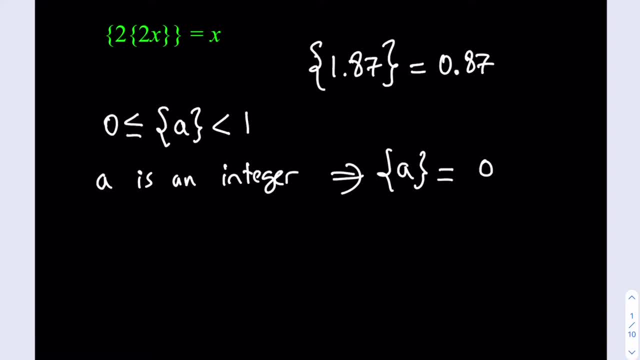 which needs to be between 0 and 1, this also shows that our x needs to be between 0 and 1.. Okay, like this. First of all, we have to start with that. Okay, so that gives us something nice. 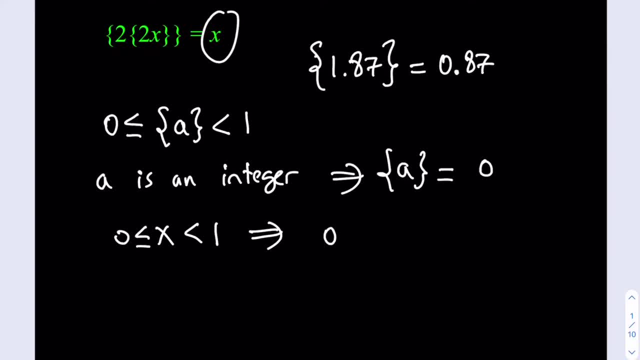 because if we multiply everything by 2 here, then we get that 2x is going to be between 0 and 2.. So I'm going to basically go off of that. But of course this is a wide range, so I kind of have to narrow it down. 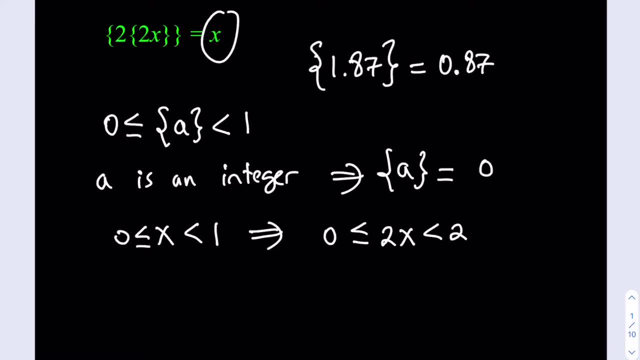 And obviously you'll realize that if x equals 0, then you know that that's going to be a solution, because the fractional part of 0 is going to be 0.. Okay, so let's go ahead and consider the first case here. Let's just call that 1.. If 2x is between 0 and 1, okay, and I can just 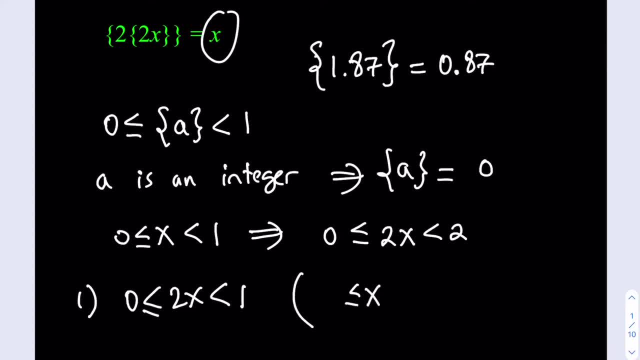 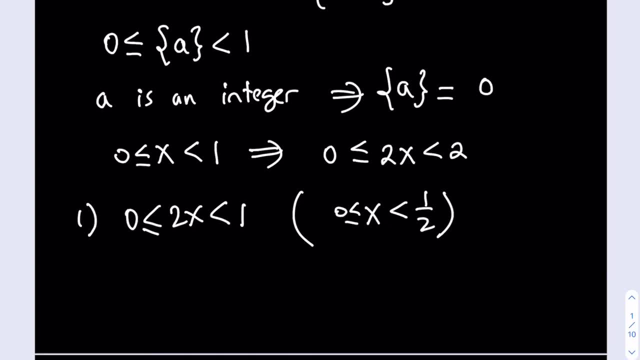 include the 0 there, meaning that x is between 0 and 1 half. right like this. then I will have that the floor value of this is going to be 0, right? So floor value of 2x is going to be 0.. 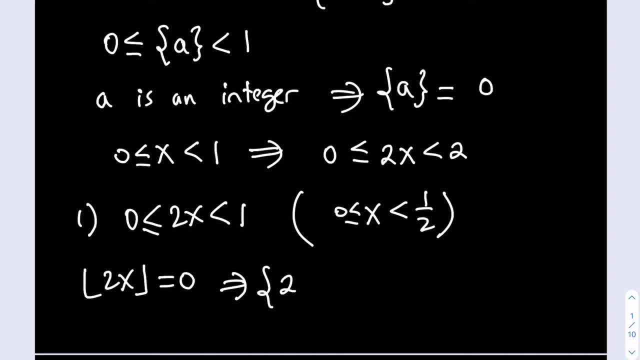 And this means that the fractional part of 2x is actually going to equal 2x minus the floor value of 2x, which is 0.. So it's just going to equal 2x, right? This is 0.. Okay, And so that means that the fractional 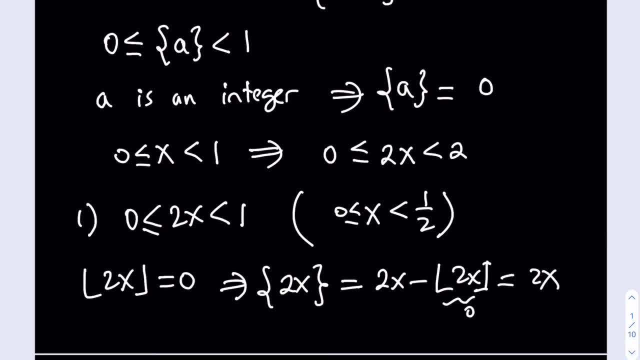 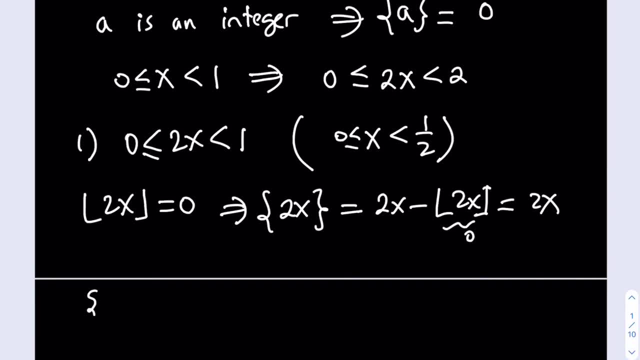 part of 2x is equal to 2x, And if I go ahead and plug that in here, then I'll be getting the floor value of 4x right. So that's going to give me the floor value of 4x is equal. 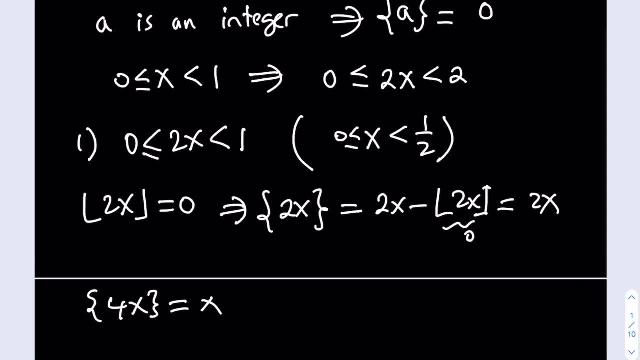 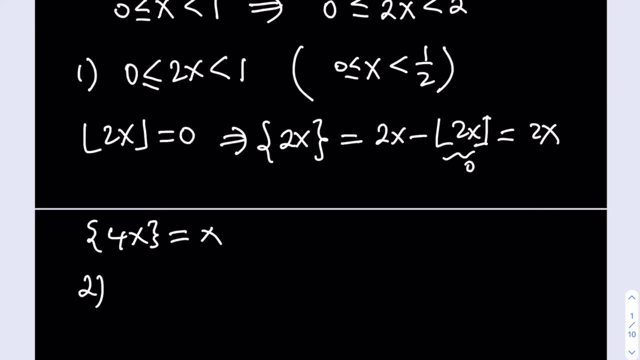 to x: Okay. so now we're gonna need to get into more cases here. So if, for example, x is between 0 and 1 half- because that was our initial assumption- right. if x is between 0 and 1 half, which means that 4x is going to be between 0 and 2, okay, so 4x is going to be between 0 and. 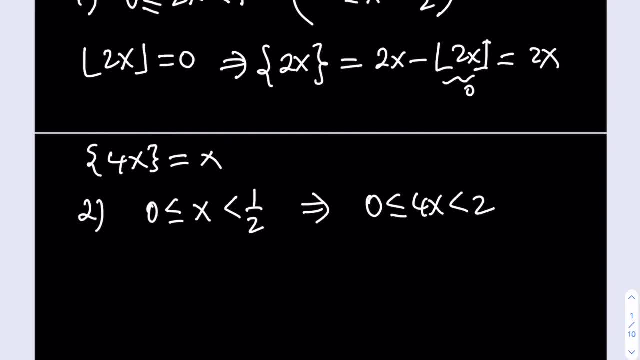 2 here. now again, this is a wide range, so i'm going to have to break it down into two pieces. first of all, i'm going to assume that 4x is between 0 and 1, meaning that x needs to be between 0 and 1. fourth now: in this case, as you know, the floor value of 4x is going to be 0 again, right? 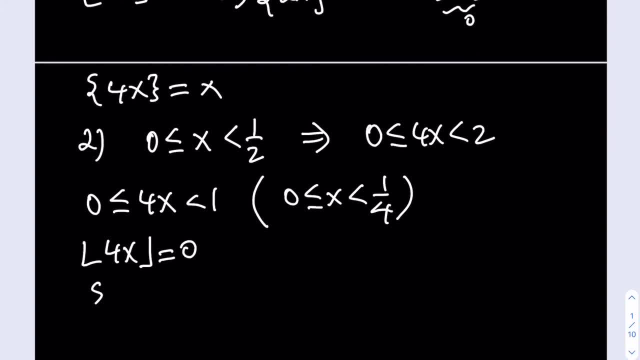 like the 2x before, and then, uh, the fractional part of 4x is going to be the same as 4x. okay, so, and we knew that the fractional part of 4x was equal to x from here, so this means that 4x. 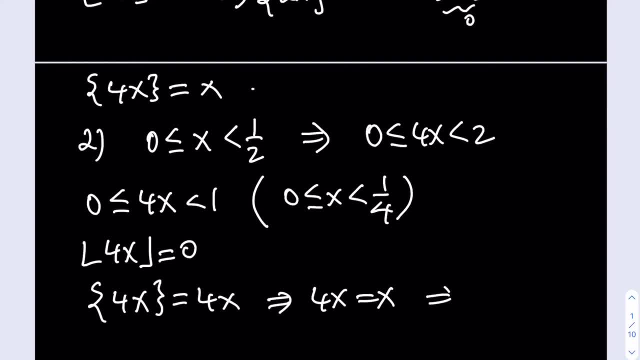 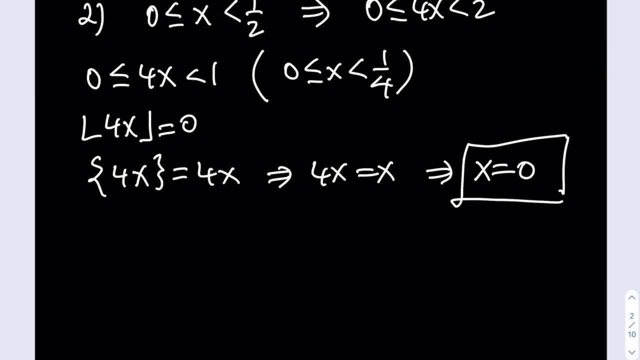 is equal to x, meaning that 3x is equal to 0. so, and that means that x equals 0. so we arrived our first solution here, starting with the assumption that x is between 0 and 1 half. okay. now the next case we're going to look at is going to be: 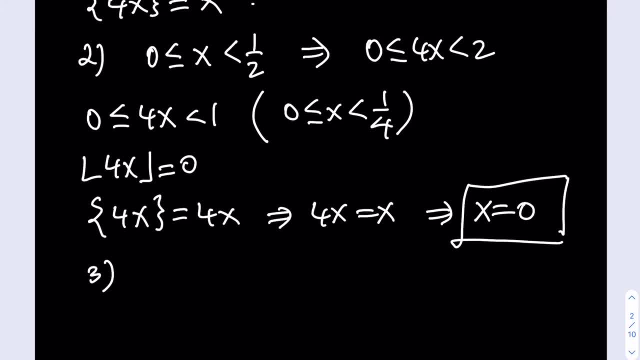 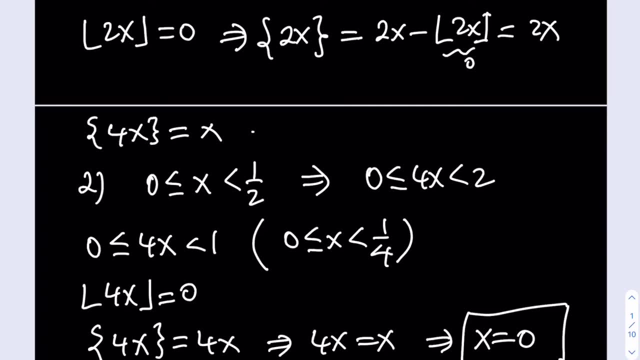 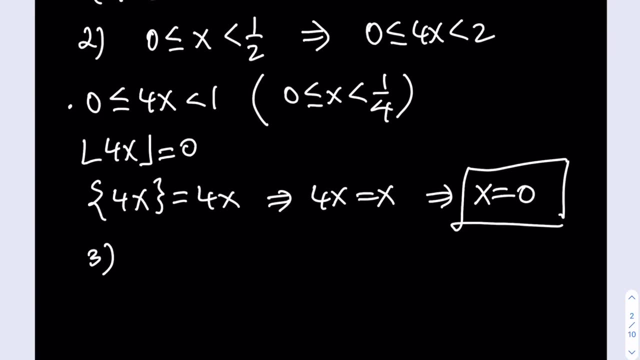 because, remember, we had said that 4x between being between: uh, where did we write that? okay, 4x being between 0 and 2 is a wide range. so we broke it down. we first said that, okay, we wanted 1 and 1. now we want it to be between 1 and 2. okay, so 4x is going to be between 1 and 2, meaning that 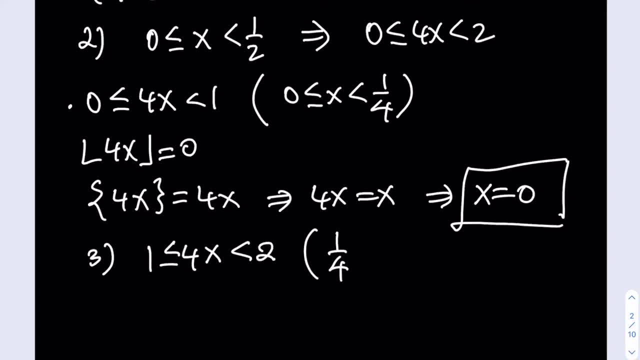 x is not going to be between one-fourth and one-half. okay, all right, that's what it means. now, if uh 4x is between 1 and 2, then the floor value of 4x is going to be, by the way, the floor. 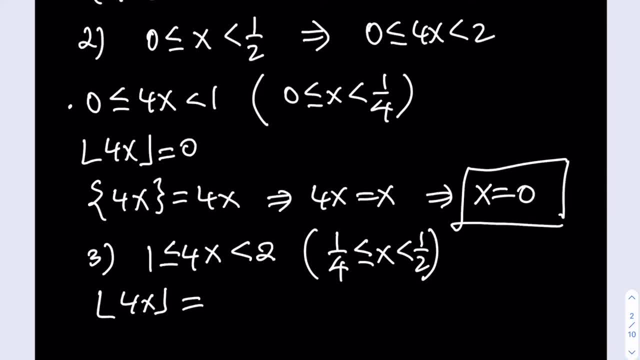 value is the same as the greatest integer function, and there are different notations, some, uh, sometimes as this one, or even this one, but they basically all mean the same thing: the integer part of 4x. okay, so in this case, it's going to equal 1, okay, meaning that the fractional part of 4x. 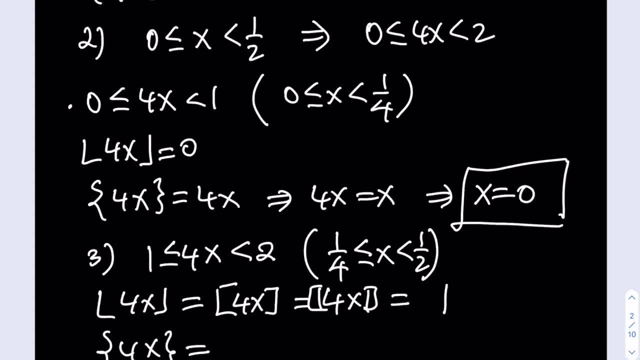 is going to be the fractional part of 4x is going to be 1 less than 4x. okay, and why is that happening? because, if you remember, we define the fractional part of a number as the number itself minus its integer part, which is 1 in this case. that's why we're subtracting 1 from the 4x. 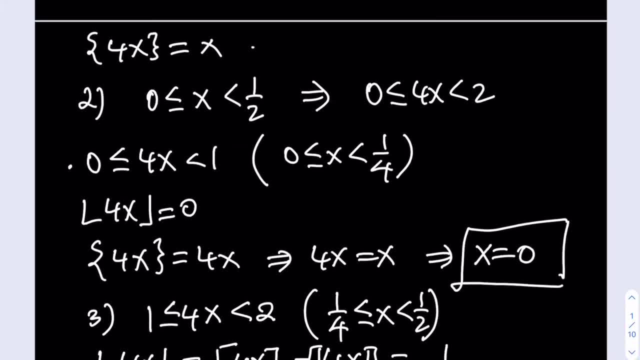 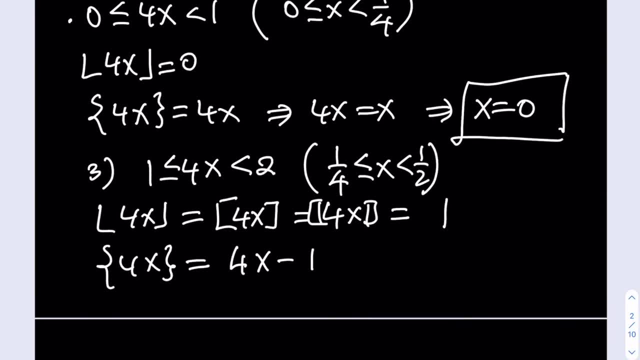 and we know that if you go back here, we knew that the fractional part of 4x is equal to x. right, and so here we're going to set the 4x minus 1- okay, is equal to 1 in this case. okay, because 4x is between 1 and 2, so that's going to equal 1 from here and this. 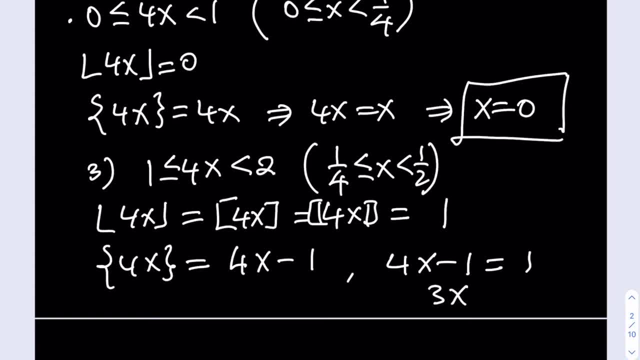 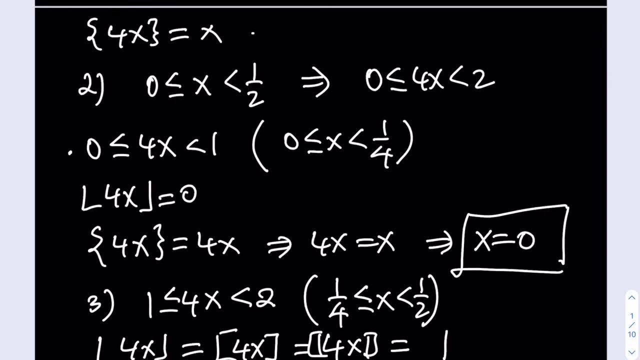 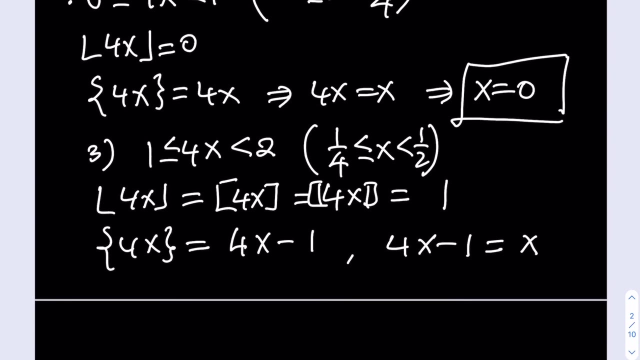 means that 3x is equal to- I'm sorry, this is equal, not 1. it should equal x. okay, so this should equal x, because we had our expression here that the floor value of- I'm sorry, the integer- what am I saying? fractional part of 4x is equal to x, and here we found that the floor value of 4x is 1. therefore, this is going to equal. 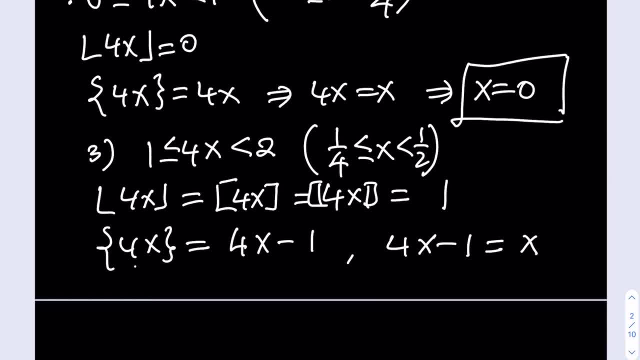 x. okay, so 4x minus 1 is equal to x, meaning that 3x is equal to 1, meaning that x is equal to 1 third. okay, so, basically, and notice that 1 third is actually between 1 fourth and 1 half, so it 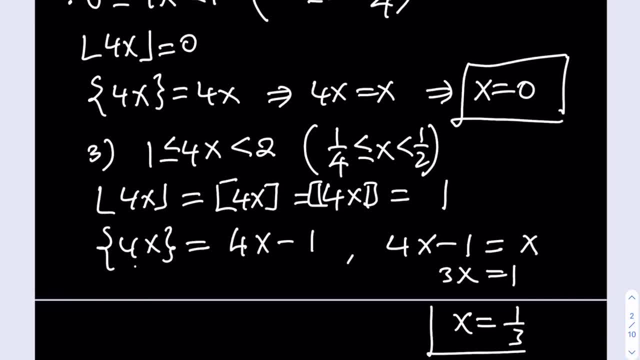 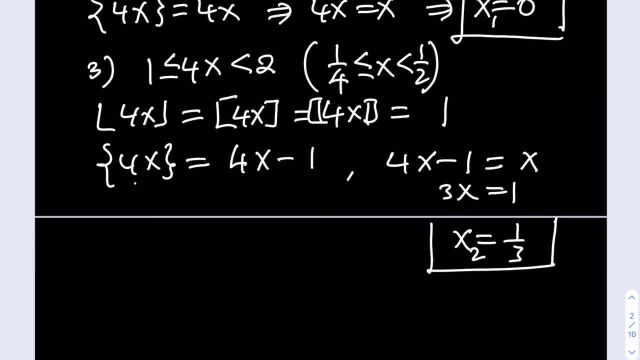 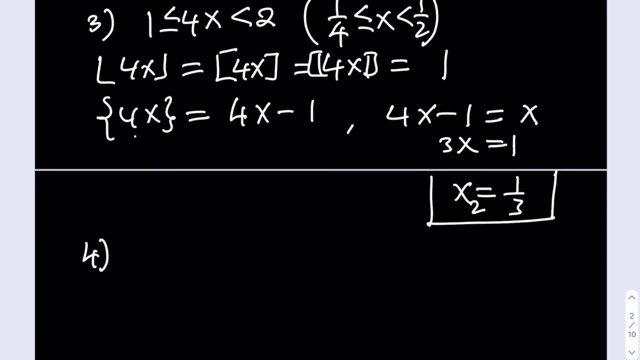 actually satisfies our equation, so we're going to take it as our second solution. okay, so i'm going to call this x1 and i'm going to call this x2 and we'll just continue with more cases. okay, so number four. what i'm going to look at is, if you remember, we had assumed that the 2x is between 0 and 2. 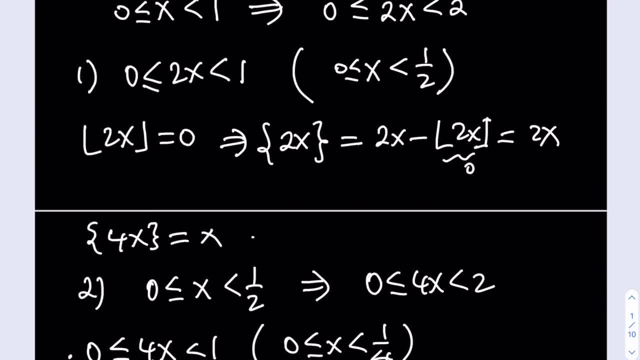 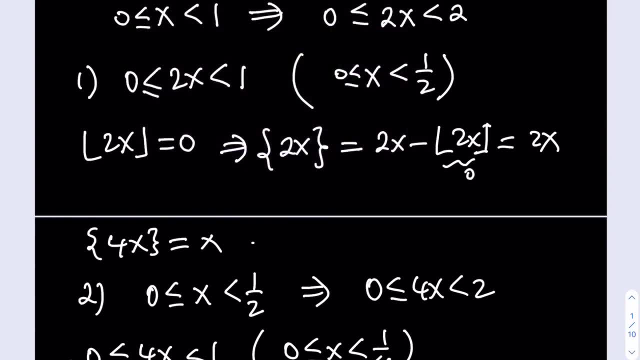 at the very beginning, right at the very beginning, our assumption was that 2x is between 0 and 2, but now we used the 0 and 1 case. now we're going to look at that between 1 and 2. okay, so now 2x is. 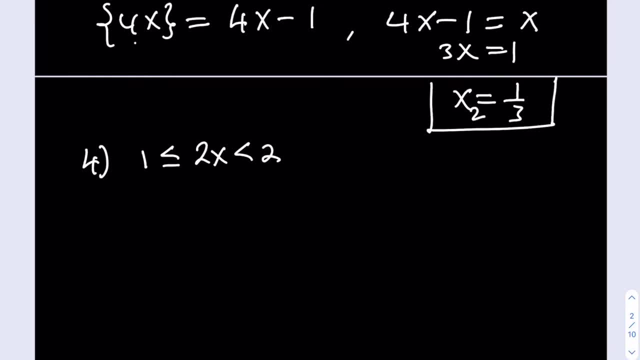 going to be between 1 and 2. in this case, it means that x is going to be between 1 half and 1. okay, and from here the floor value of 2x is actually going to be 1, meaning that the fractional part of 2x is going to be 1 less than 2x right by our general formula. 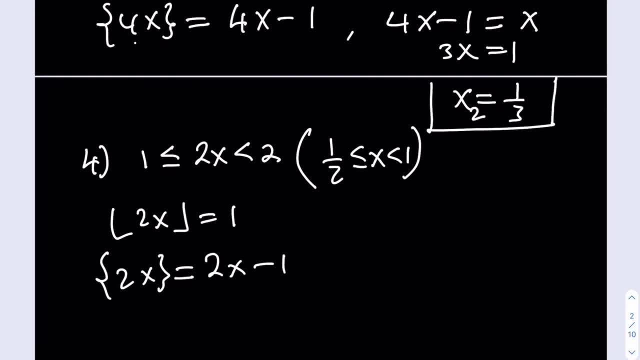 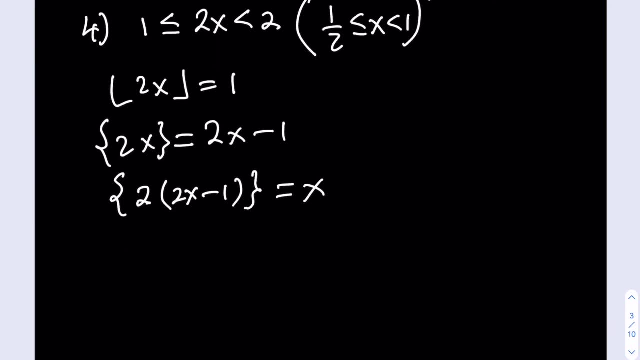 so remember, we had a fractional part and then inside there was another fractional part, and this means that the fractional part of 2 times the fractional part of 2x, which is equal to 2x minus 1, here right, equal to x, and then this is going to give us the fractional part of 4x minus 2. 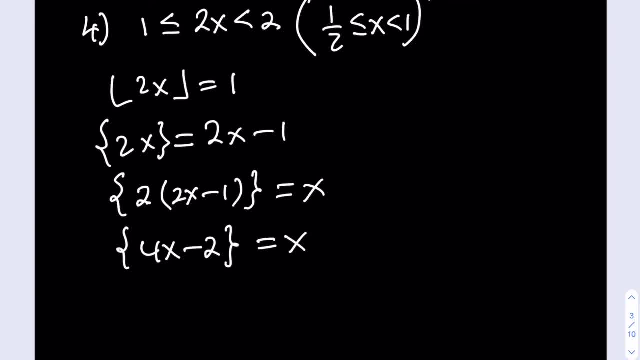 being equal to x. now we know that x is between 1 and 1 half and 1, right, so let's go ahead and write that down: x is between 1 half and 1, okay, and that means that if you multiply everything by 4, 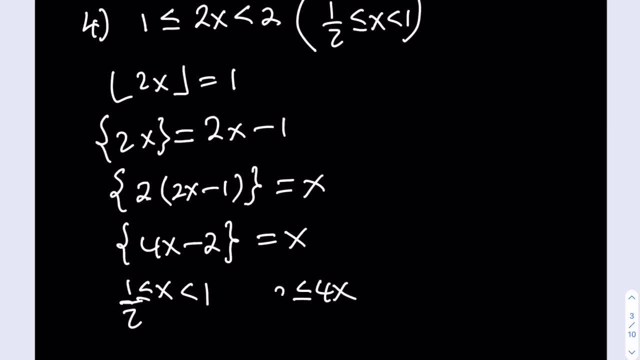 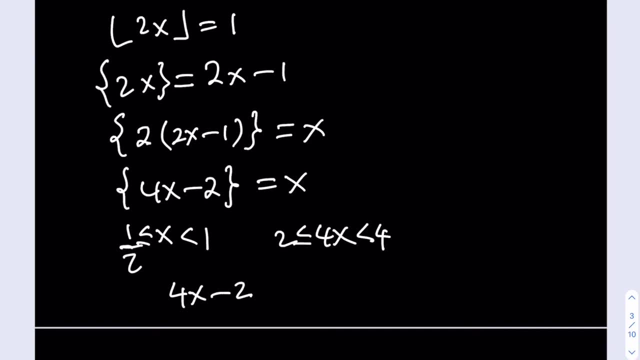 4x is going to be between 2 and 4. okay, so let's subtract 2 from both sides. that means 4x minus 2 is going to be between 0 and 2. now the reason why i'm looking into 4x minus 2 is because i got this: 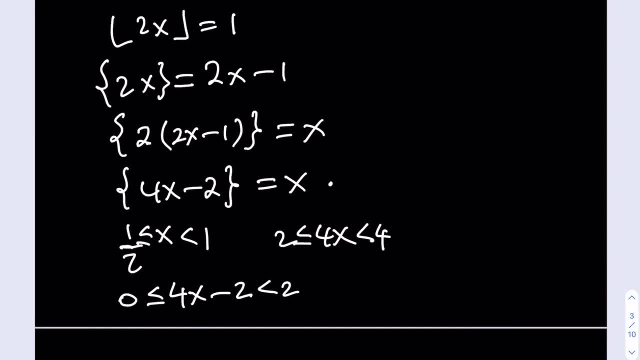 equation here. so i kind of need to know the the floor value of 4x minus 2 is going to be between 0 and 2, so that i can talk about the fractional part of 4x minus 2 here. okay, so again we're going. 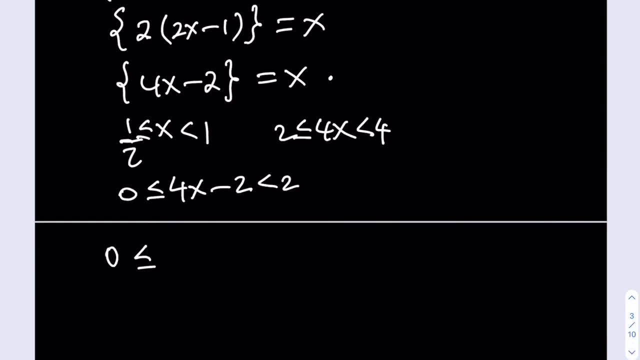 to be splitting it up into two pieces, and one of them is going to be between 0 and 1. okay, this. this means that 4x is going to be between 2 and 3 and that means that x is between 1 half and 3. fourths: 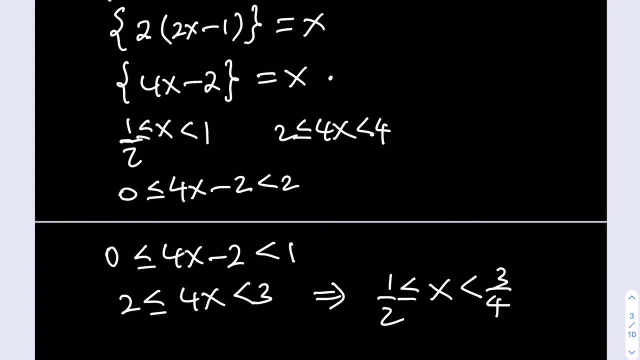 okay, now. now, what does this mean? for the 4x minus 2 to be between 0 and 1, right? so we're going to be splitting it up into two pieces and one? it means that its floor value is going to be 0, right? and 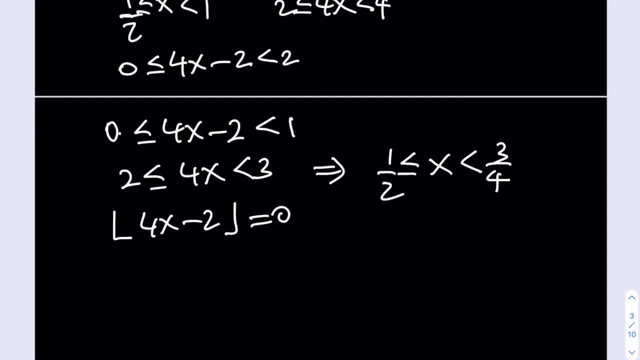 that means that the fractional part of 4x minus 2 is going to be the same thing as 4x minus 2. okay, so it's going to be the exact same thing, and if you knew that the fractional part of 4x minus 2. 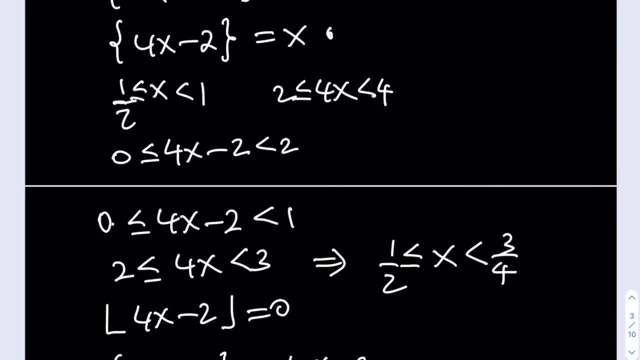 was equal to x from here. right, so we're just going to go ahead and set it equal to x, and from here we're going to be getting 3x equal to 4x minus 2, and we're going to be getting 3x equal to. 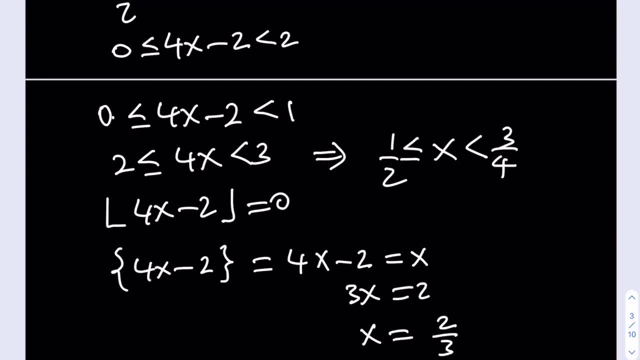 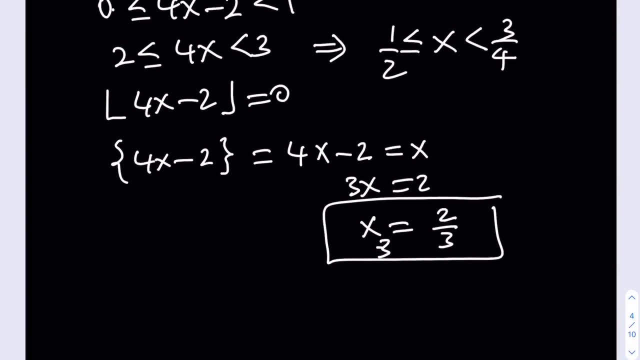 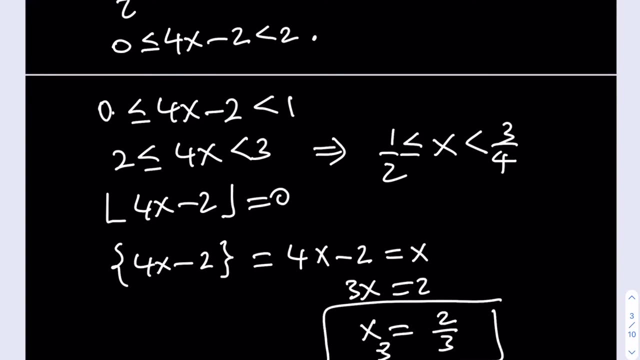 2 and x equals 2 thirds, and that's going to be our third solution, okay, and we're going to be looking at one more case, and that is going to come from here. if you remember, we got that 4x minus 2 is between 0 and 2, and we looked at this one. now we're going to be looking at the other piece, which 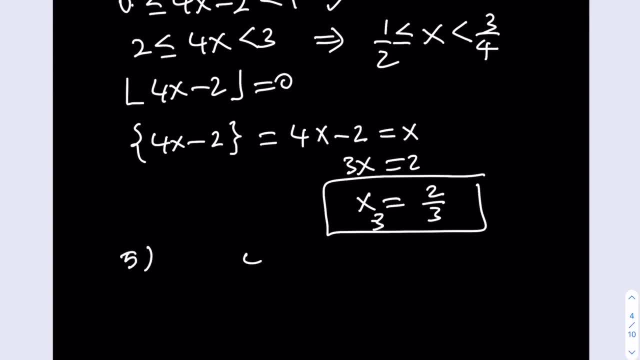 is when the 4x minus 2 is between 1 and 2. okay, all right. so we always have to make sure that it's between two consecutive integers so that we can easily calculate the floor value, and this means that x needs to be obviously between 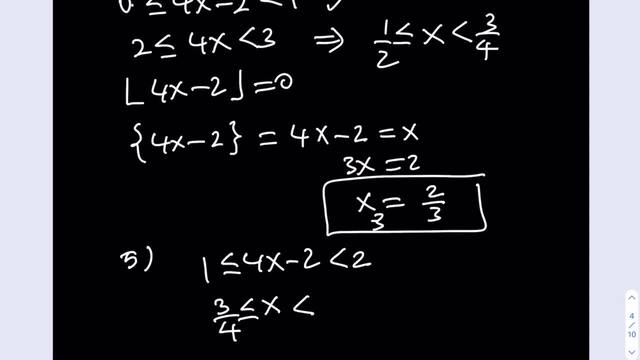 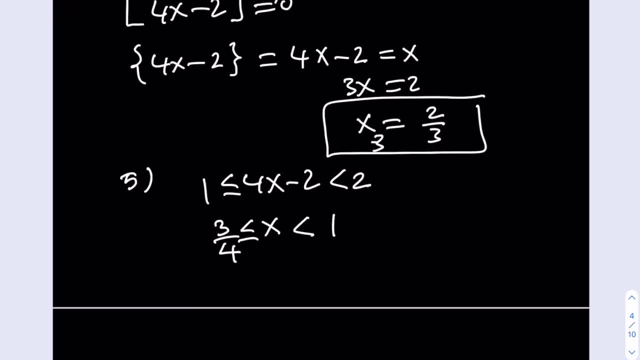 3 fourths and 1. okay, if you add 2 to both sides, i mean everything- and then divide by 4, okay. so we're gonna proceed from here. because the 4x minus 2 is between 1 and 2, its floor value is going to. 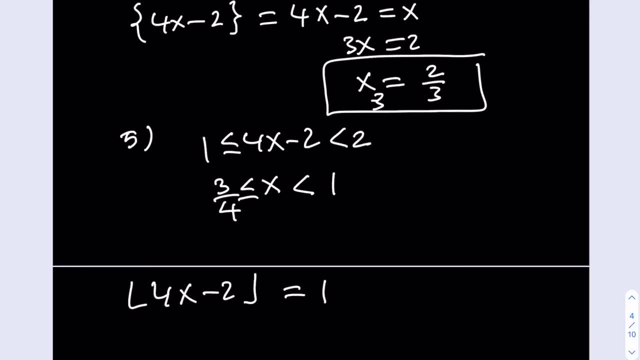 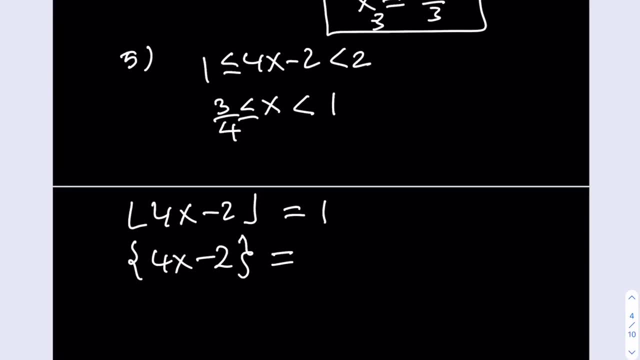 equal 1 from here, which means that the integer- i mean the fractional part of this guy here- is going to be one less, because it's always less by the integer part, right. so that's going to equal 4x minus 2 minus 1, which. 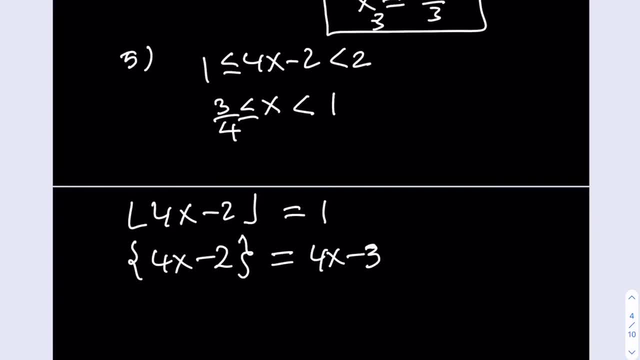 is 4x minus 3. so in other words, if the floor value of something is 1, then its fractional part is going to be 1 less than, for example, let's think about 1.5. the fractional part of 1.5 is 1.5 minus 1, which is 0.5. okay, and from here 4x minus 3. 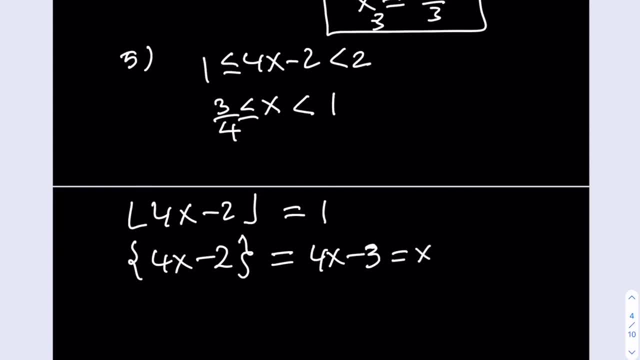 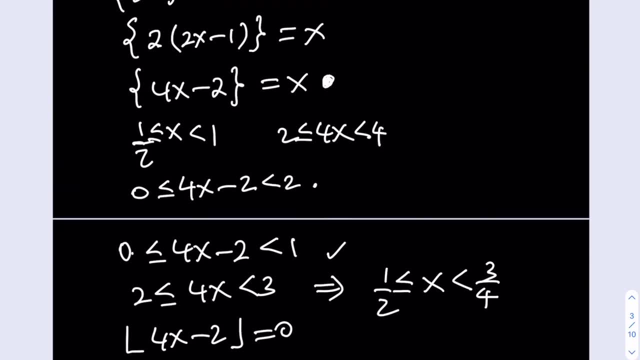 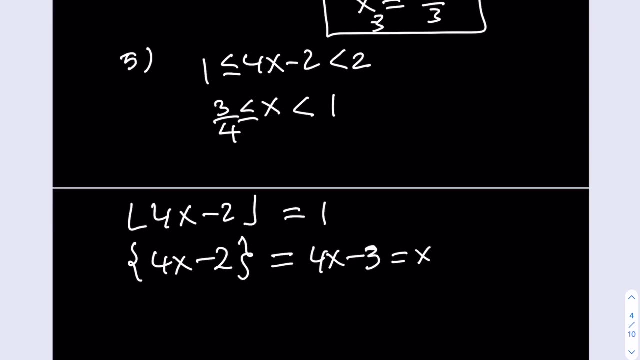 is equal to x because, if you remember, we said that the where did we say that? okay, right here. okay, we said that the fractional part of 4x minus 2 is equal to x, because that's what came from our original equation, and now we're going to set it equal to x here, like this: okay, so this gives us a. 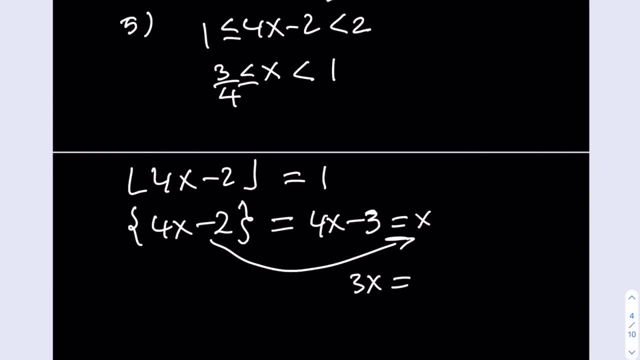 really nice equation because i can see that the fractional part of 4x minus 2 is equal to x, and subtract x, this gives me 3x equals 3 and x equals 1, and that's going to be our fourth solution: x to x. fourth is one. let's go ahead and write down all the solutions here. i'm going to go ahead and list.